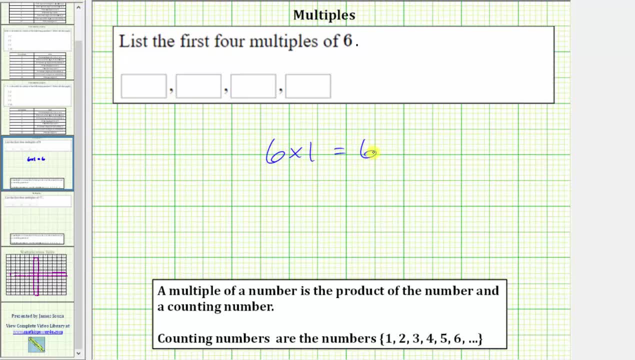 is six times one, which equals six. The first multiple of any number is a number itself. The next multiple is six times two, which is 12.. The next multiple is six times three, which equals 18.. And the fourth multiple of six is six times four. 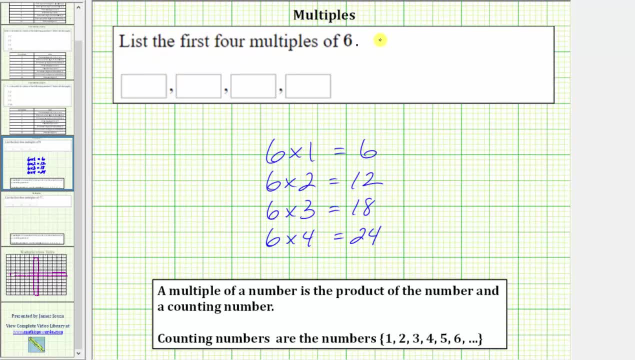 which equals 24.. The first four multiples of six are: six comma 12 comma, 18 comma 24.. You may also notice another pattern in the multiples of six. Notice: six plus six equals 12.. 12 plus six equals 18.. 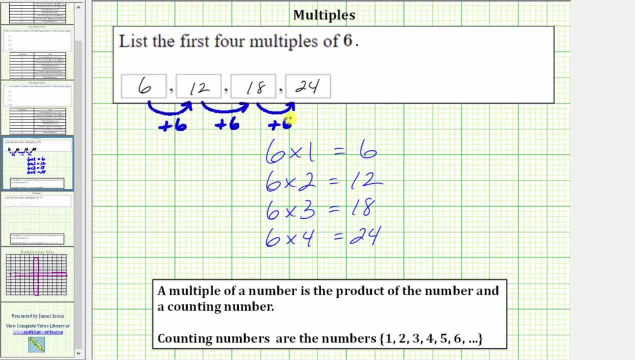 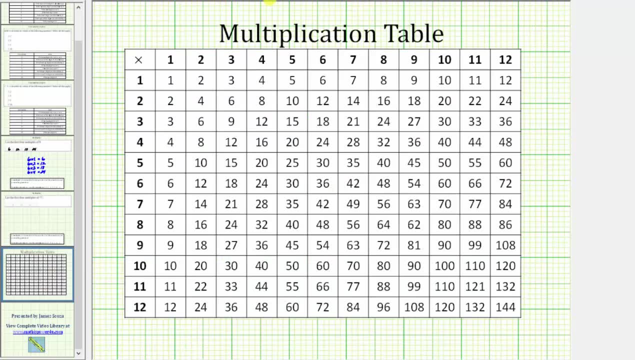 And 18 plus six equals 24.. We can also find the multiples of six in a standard multiplication table. Here we have a typical 12 by 12 multiplication table. The row and column containing six also shows multiples of six. Notice: this row gives us multiples of six. 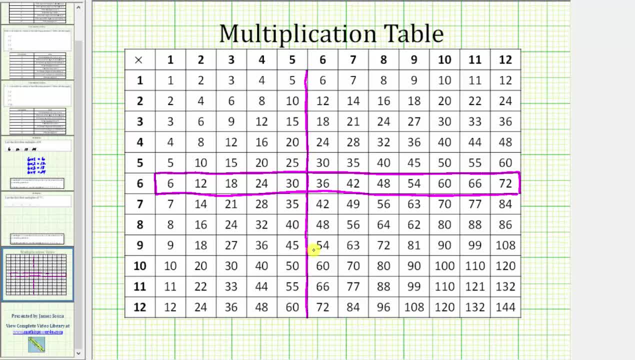 And this column also gives us multiples of six. In fact, the row and column give us the first 12 multiples of six. Here we have six: 12,, 18,, 24, and so on. In this row, in this column, we have six: 12,, 18,, 24,. 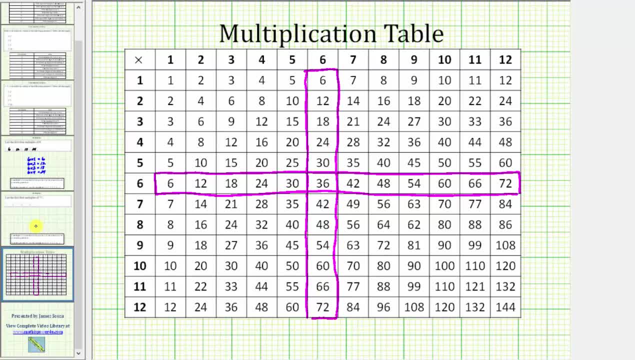 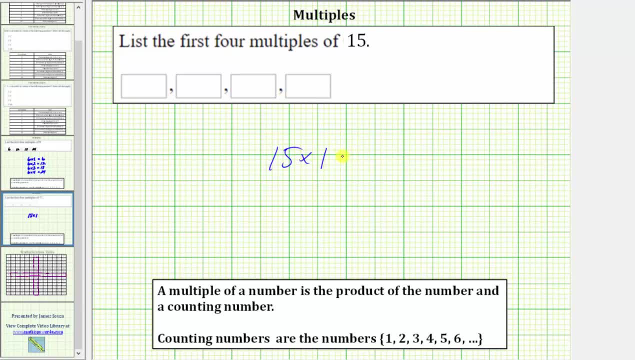 and so on as well. Let's look at one more example. Here we're asked to list the first four multiples of 15.. The first multiple of 15 is 15 times one, which is 15.. The next multiple is 15 times two, which equals 15.. 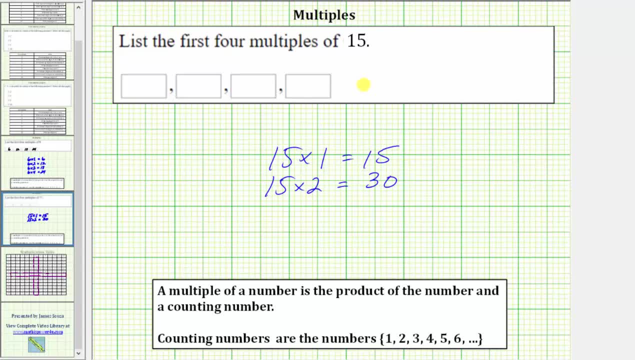 That's 15 times two 2,, which is equal to 30.. The third multiple of 15 is 15 times 3,, which is equal to 45.. And the fourth multiple of 15 is 15 times 4, which equals 60.. The first four multiples. 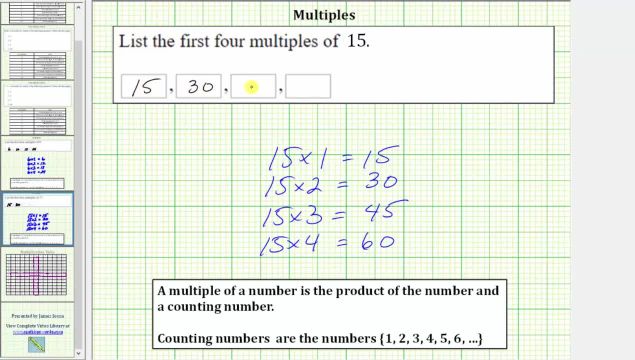 of 15 are 15, 30,, 45,, 60. And again, there's also a pattern of addition here: 15 plus 15 equals 30. 30 plus 15 equals 45. And 45 plus 15 is equal to 60.. I hope you found this helpful.